primarily made of just two ingredients. The atmosphere is made of a whole bunch of different elements, but most of it is just nitrogen and oxygen. These two elements account for 99% of the volume of the atmosphere, with most of the remainder being argon. 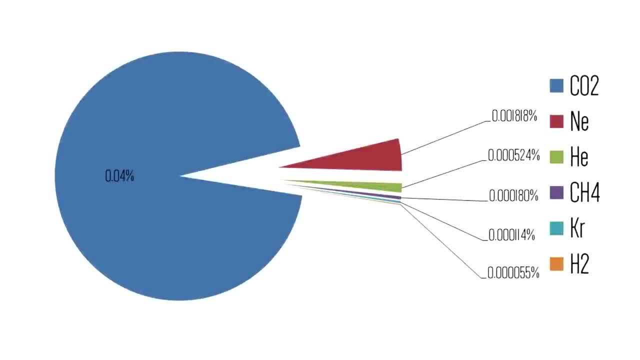 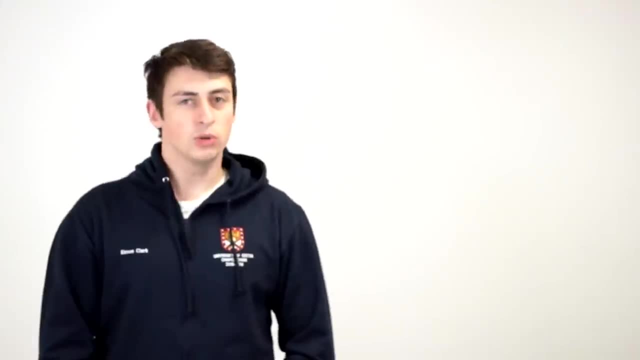 The last few hundredths of a percent are mostly carbon dioxide, with neon, hydrogen, helium, methane and krypton all making guest appearances. It's also worth noting that, at any given time, about a quarter of a percent of the atmosphere's mass is water vapor, which goes some way to 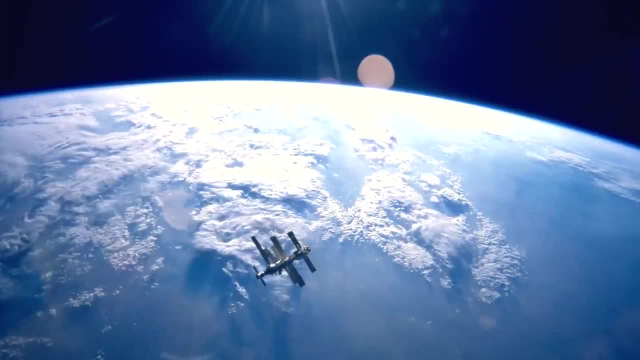 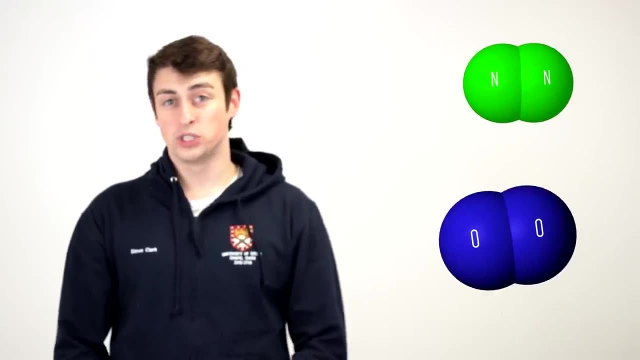 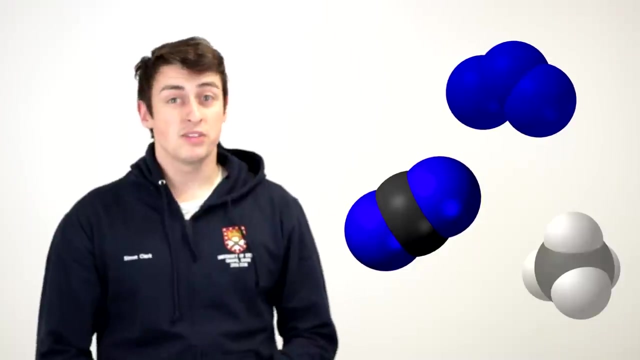 explaining why the atmosphere looks so cloudy from space. Notice that 99% of the atmosphere is either N2 or O2, the stable molecular forms of nitrogen and oxygen, both of which have two atoms apiece. These gases, such as ozone, carbon dioxide and methane, all have more than two atoms. 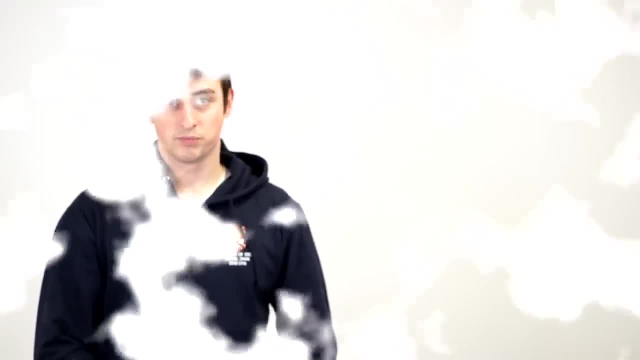 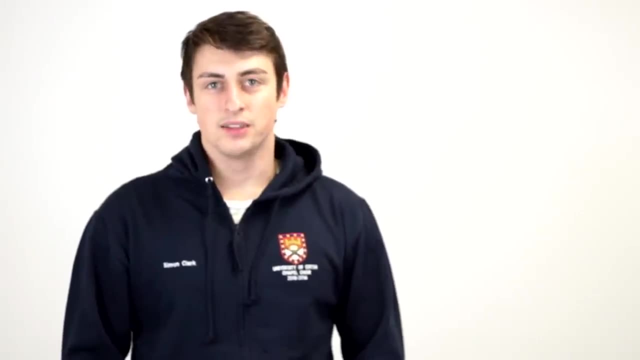 each is very significant and we're going to talk more about that in future videos. Like onions, like ogres, the atmosphere is made of many layers And these are layers which humans have defined but have a physical, non-arbitrary basis And the most common way. 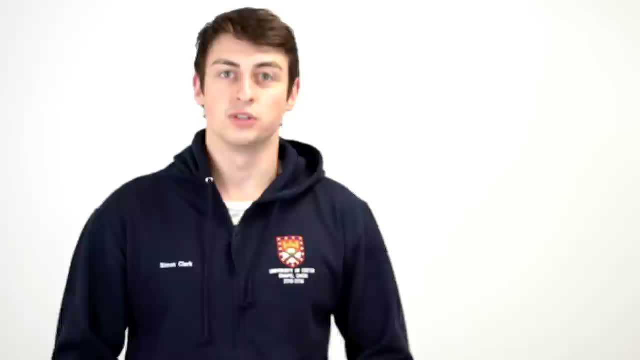 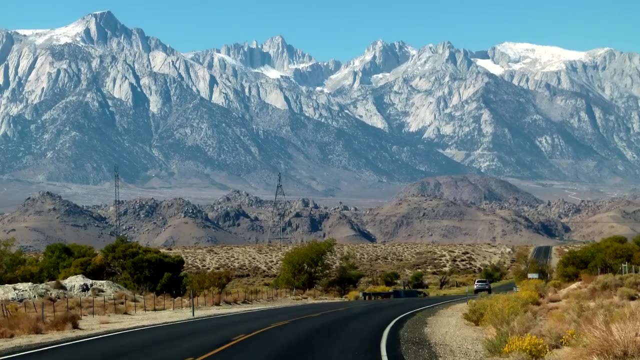 in which we define these layers is to use the temperature profile in the vertical, so seeing how temperatures change with altitude Here at the surface, we're very familiar with the fact that the higher you go up, the colder it gets. This is why mountaineers who are climbing 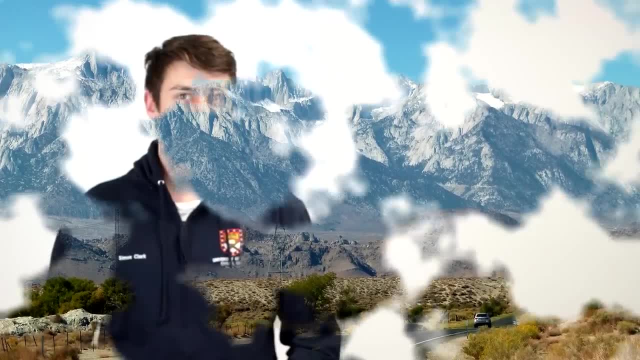 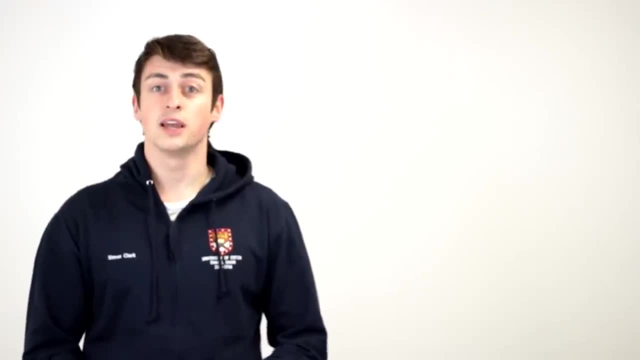 Everest have to wear so many different insulating layers instead of shorts and flip-flops. So we define the bottom layer of the atmosphere, the layer in which we live, to be where temperatures decrease with altitude, and we call this layer the troposphere. 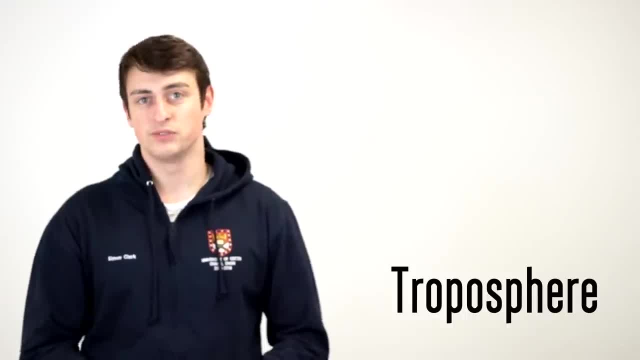 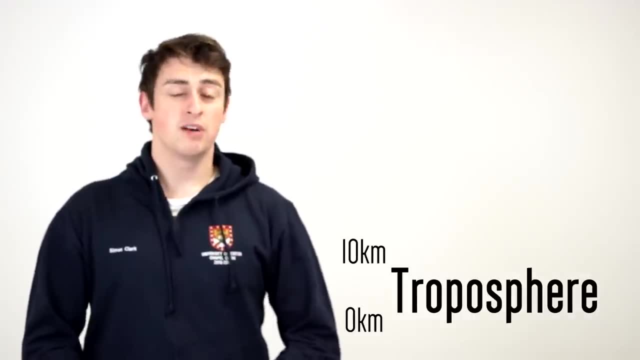 And the troposphere accounts for about 70% of the whole mass of the atmosphere, but it doesn't extend all that far up. Temperatures decrease from the surface up to about 10 km in altitude, where they reach a minimum of about minus 50 or 60 degrees Celsius. But here the 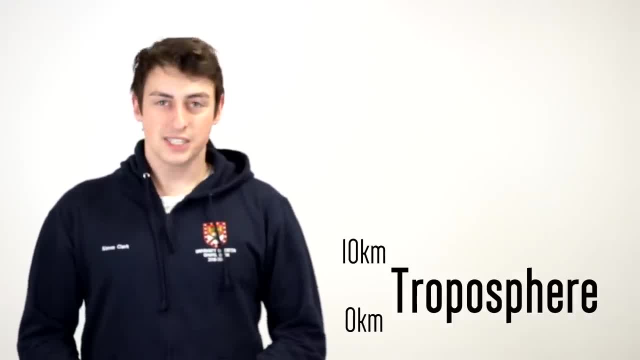 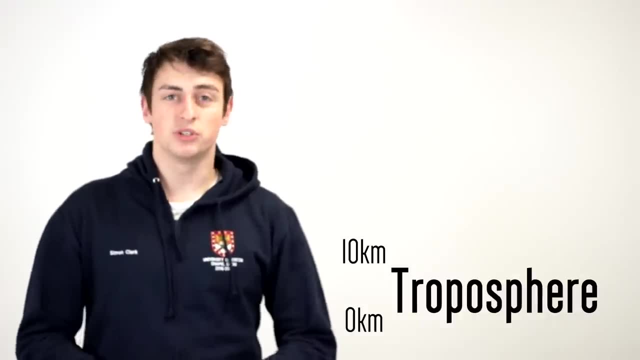 atmosphere starts to do something kind of strange. Temperatures stay the same for a few kilometers and then, as you get higher, they start to increase, And they increase up to a maximum of about 0 degrees Celsius at 50 km or so in altitude, And beyond this point the temperature starts to decrease again as you go higher up. Now, that layer between 10 km and 50 km in altitude is what we call the stratosphere, and it accounts for almost the entirety of the remaining mass of the atmosphere. Above it you have the mesosphere stretching from about 50 to 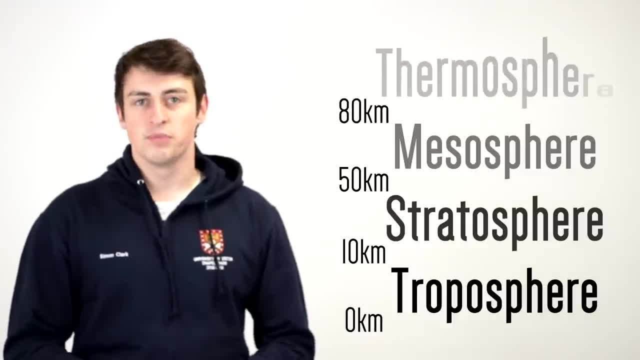 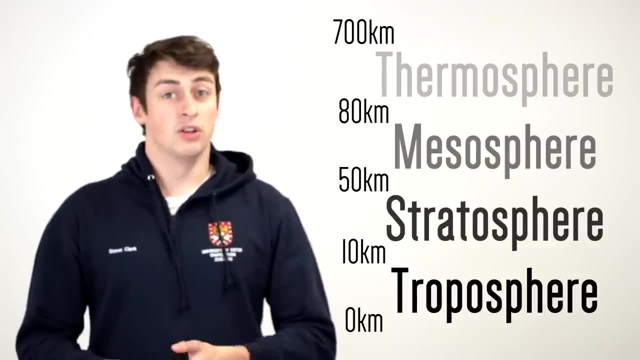 80 km in altitude and above the mesosphere, you have the thermosphere, beyond which the atmospheric density is so low that you're basically in the vacuum of space, Although it's worth pointing out that the atmospheric density is so low here that all it takes is for 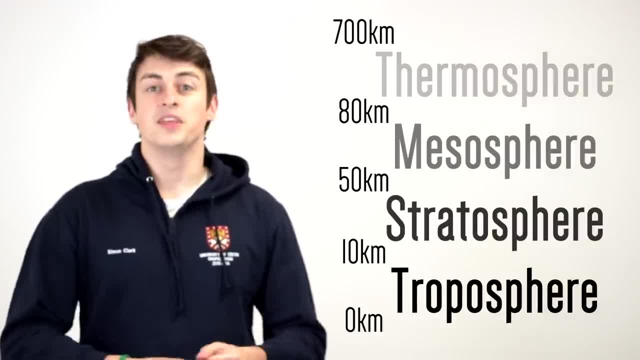 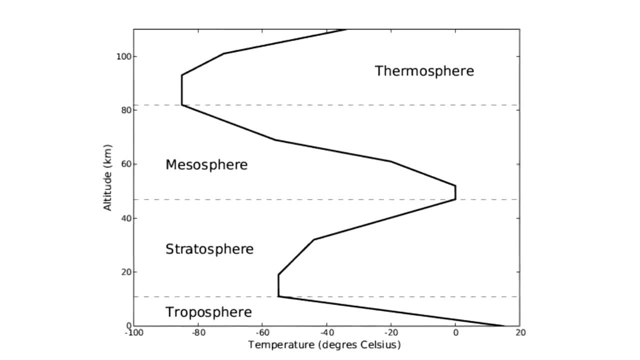 a few atoms in the layer to be ionized by solar radiation, and the temperature- the average temperature of the whole layer shoots up, which is why these graphs look a little bit strange. When we talk about the atmosphere, what most of the time we mean is the troposphere.